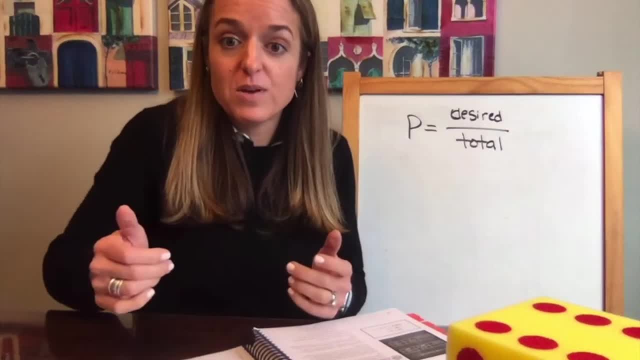 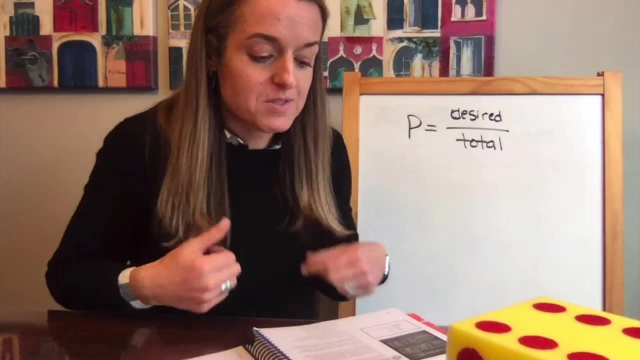 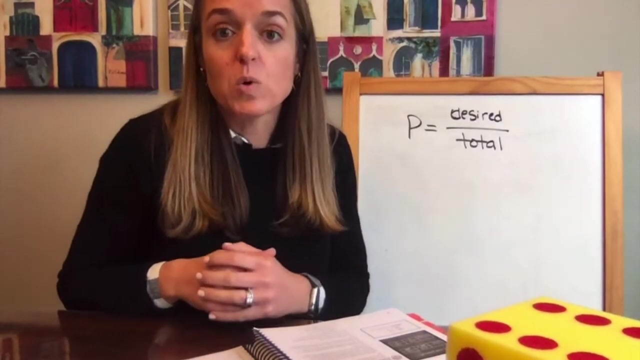 But if I have two groups, I'm going to flip a coin to see who gets it. Are the odds the same for both of you? Yes, they are right, They are the same, so they are technically fair. We're not actually going to have a treat, but what I want you guys to do is work in pairs and 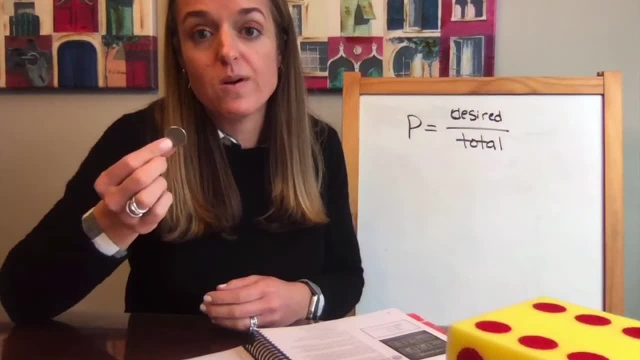 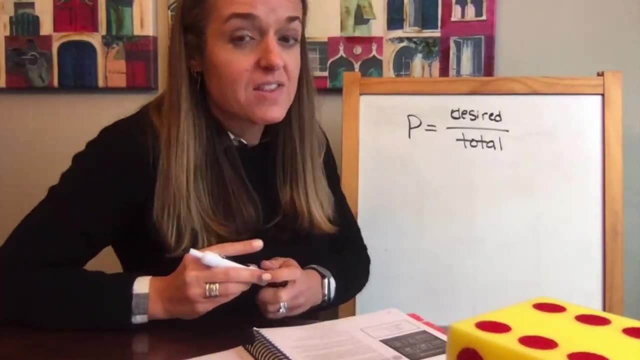 just like we did the first week of this quarter. I want you guys to flip the coin 12 times and keep track of heads versus tails. okay, Do you remember what that probability was that we would get when we flip a coin? Desire atака, Desire ataka. That's the probability. Do you remember what that probability is? 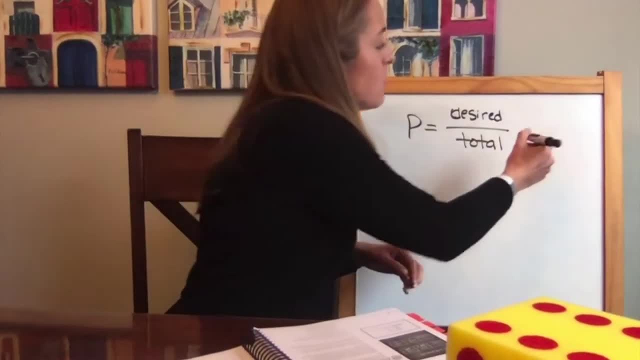 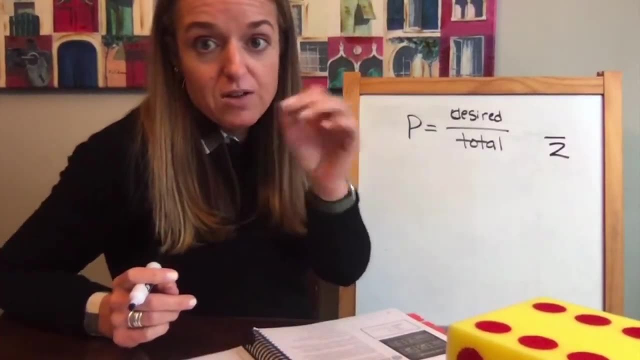 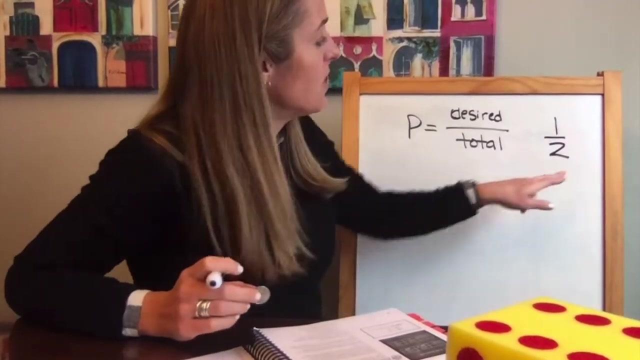 desired outcomes over total outcomes. How many total outcomes in a coin? toss Two right And you're going to choose any one of your desired outcomes, either heads or tails. So there's one desired outcome. So one over two. So let's flip the coin 12 times and see if you're, if you get. 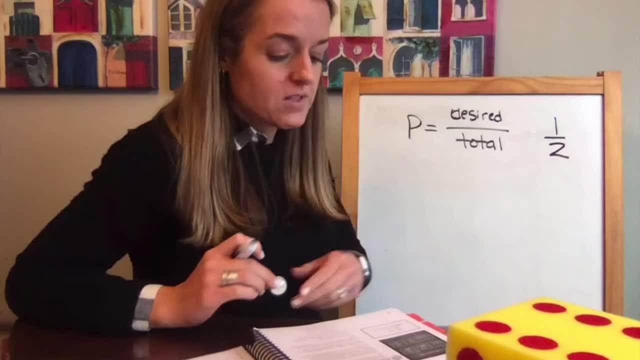 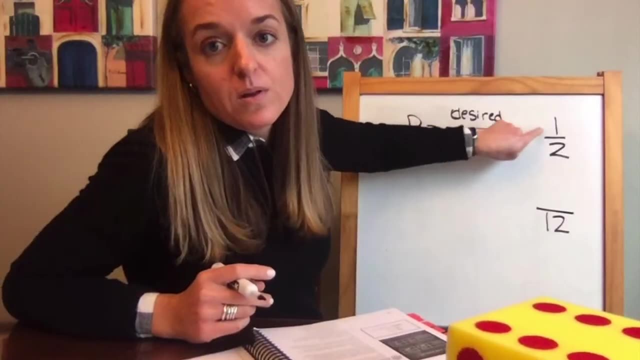 close to a one over two um coin toss. So if we're going to do 12 tosses, then what's going to be pretty close to one over two, What's going to be pretty close Six, right, Let's see if we. 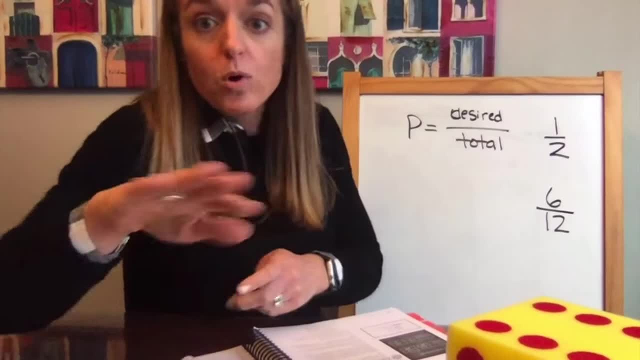 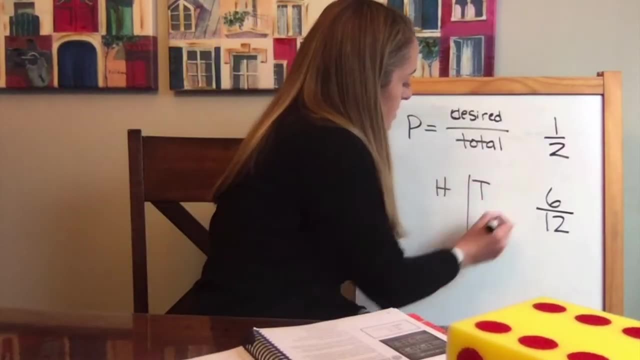 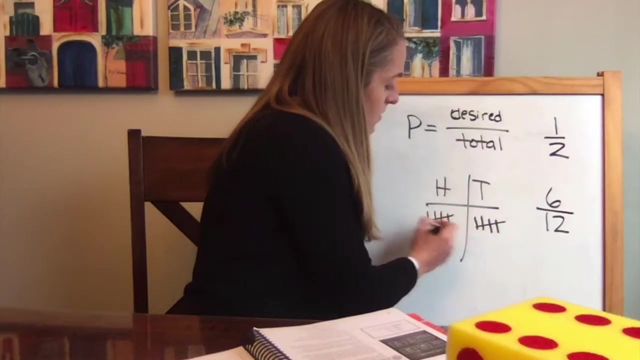 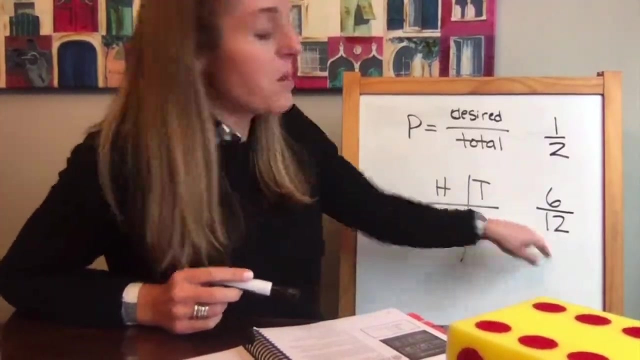 can get pretty close to six. So work in pairs. flip your coin 12 times: heads, tails, t-chart, make your hash marks Okay And see how close you get. And right now, right now, write down what your probability was. What probability did you and your partner get? 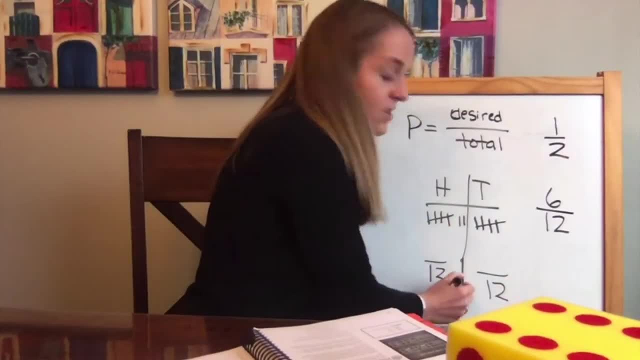 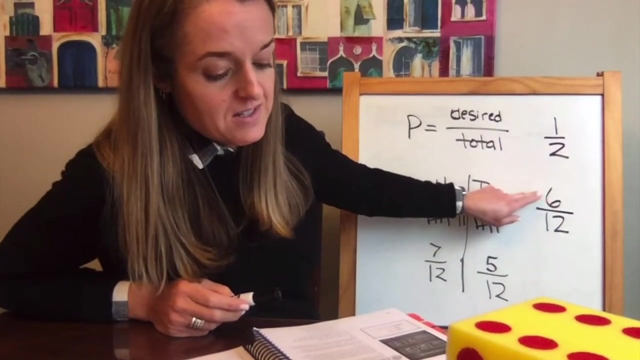 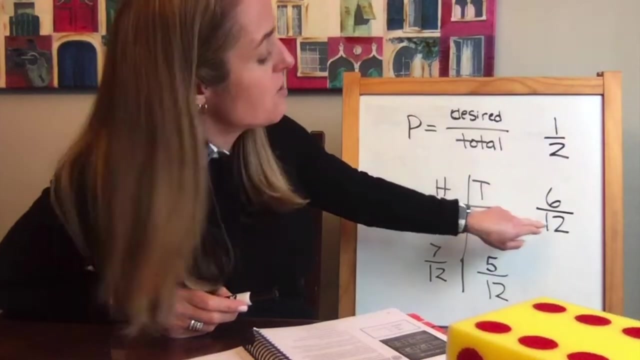 In this case I didn't actually flip the coin, but in this case I got seven heads, So seven out of 12, and five tails- five out of 12.. So that's reasonably close to six. Remind me, how can I get closer to six? I can increase the total number of outcomes, right, I can flip the. 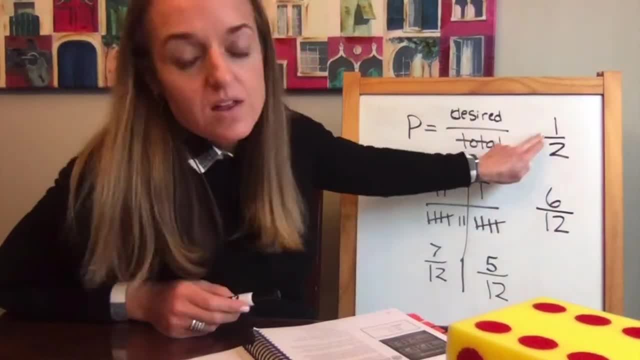 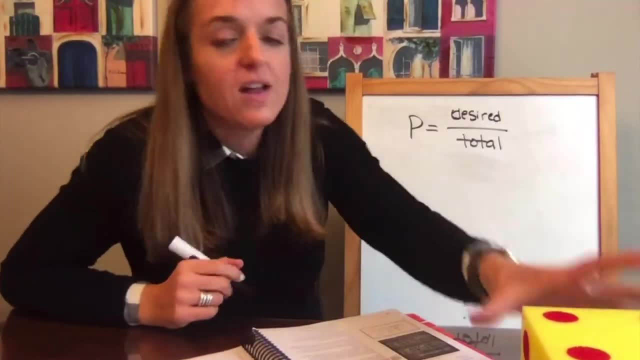 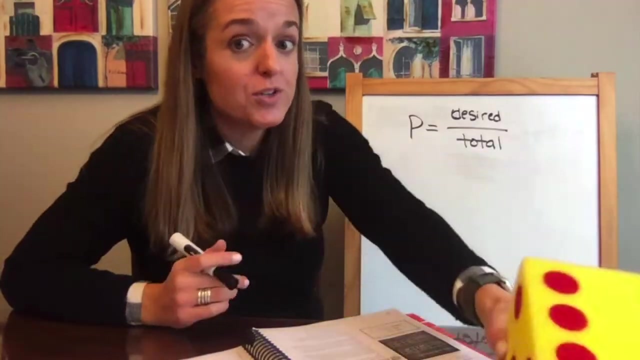 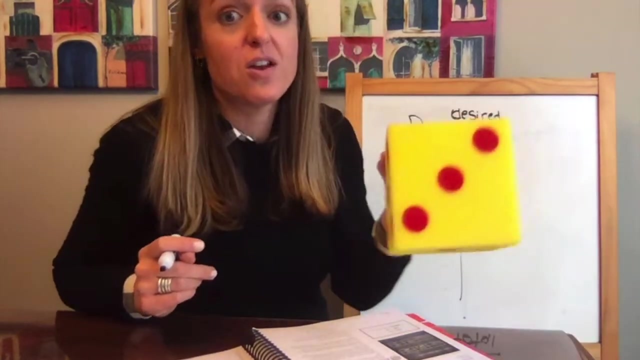 coin. Okay, The closer it's going to get to six over 12, to one half, to one out of two. Now let's change the problem. Instead of flipping a coin, what if we roll a dice? What if we say that this team will get the treat if we land on a one or a two, And this team will get the treat if we land on a three, four, five or six? 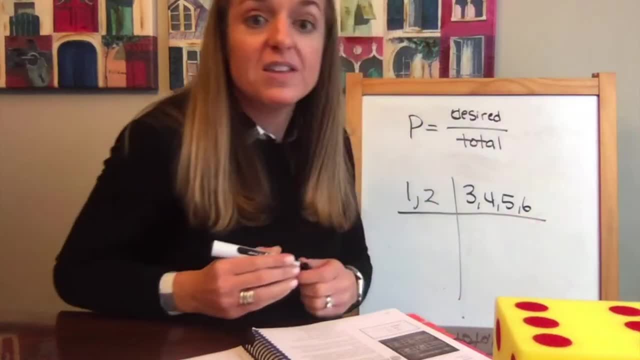 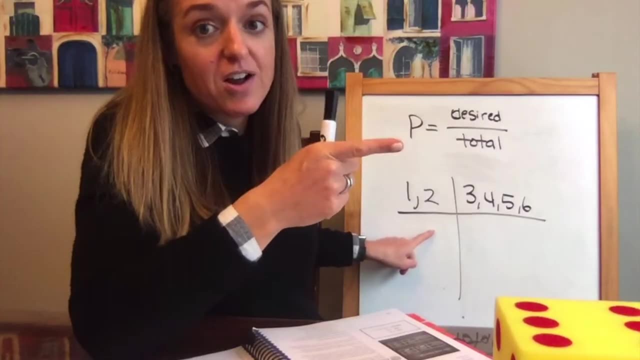 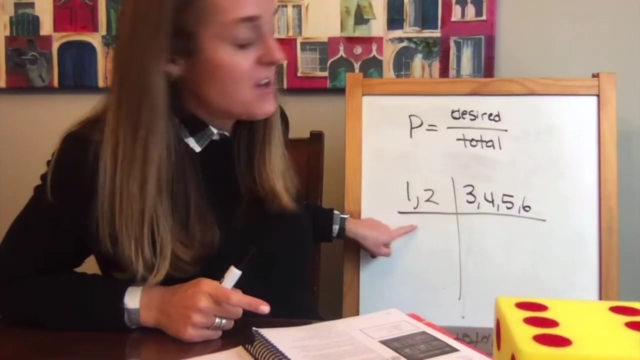 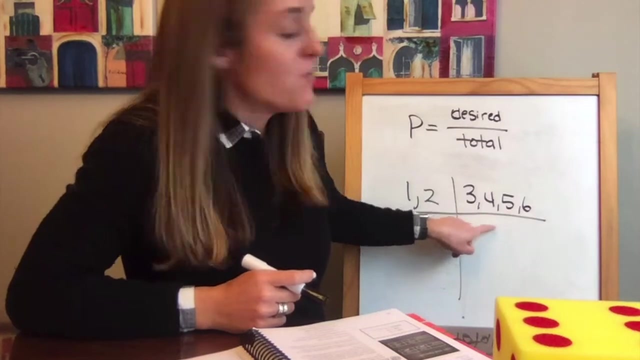 What do you think the odds are that this team is going to win the treat? You think they have a better odds, better odds or worse odds? They have worse odds because they've only got two numbers to come up. But this team they have good odds. They have much better odds of winning because they have more numbers that might be able to come up. So when we talk about odds, we're going to, we're talking about 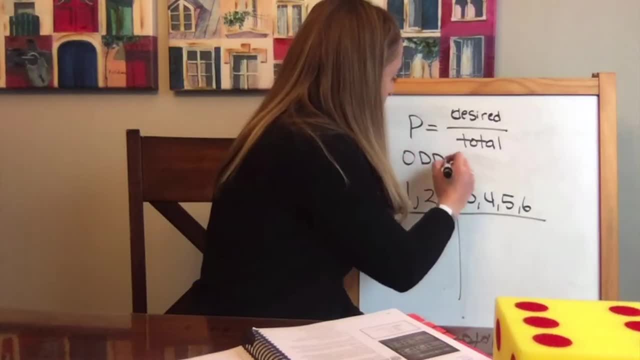 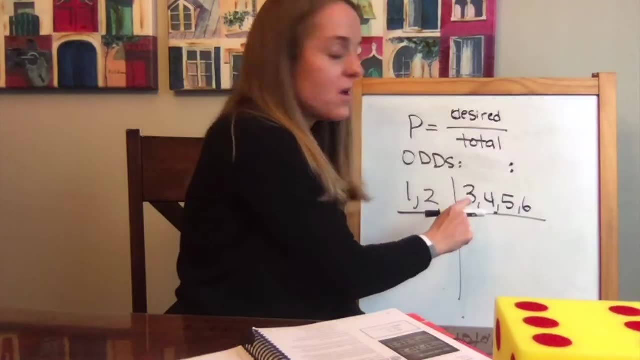 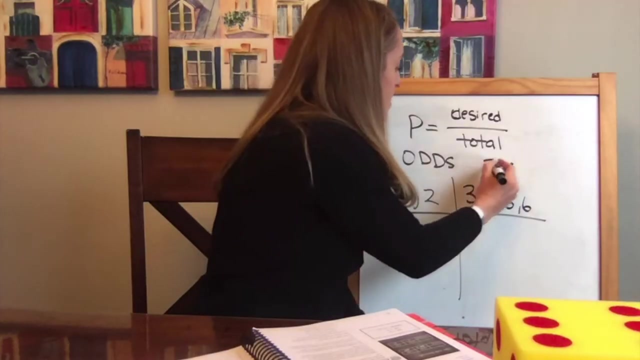 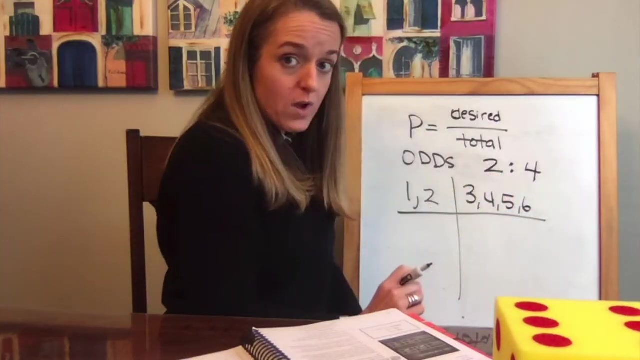 ratio And that we use a colon. So in probability we use a fraction to talk about what we're talking about, But with odds we're going to use a colon and a ratio. So here we have two outcomes to four outcomes, two to four outcomes. When we flipped a coin, our ratio was one to one, because you can either get heads. 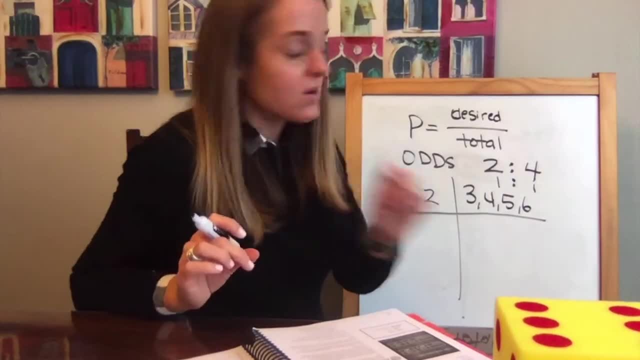 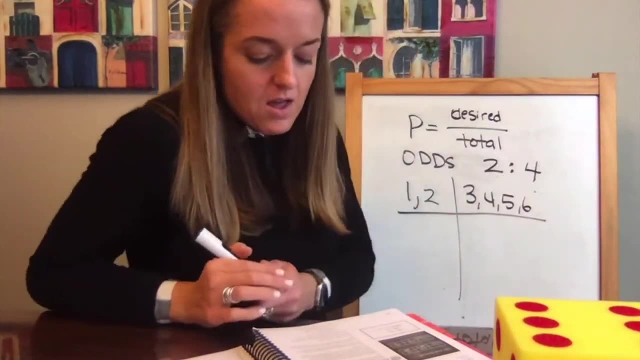 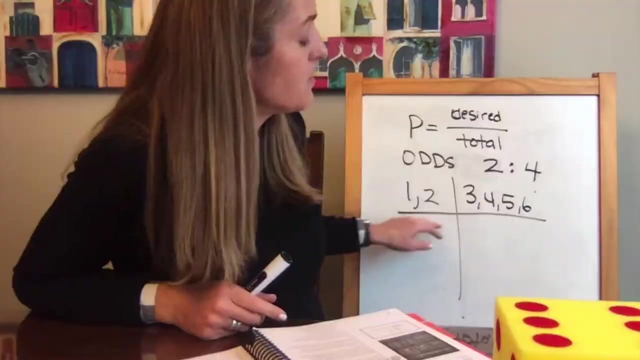 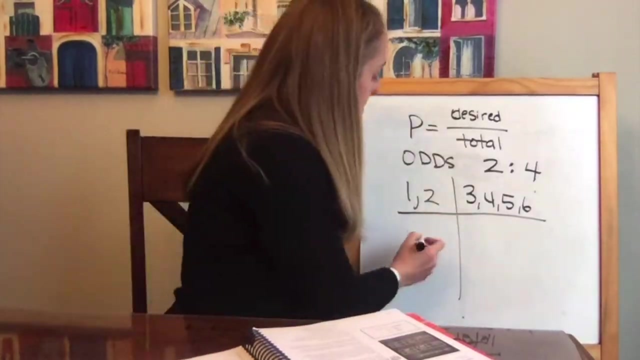 or you could get tails. Both of those was one outcome, So it was one to one. So why don't we roll the die and see? see what we get. Let's try and roll the die 12 times and see how many times each of these numbers come up. Okay, so if we roll the die, we should get something similar to: 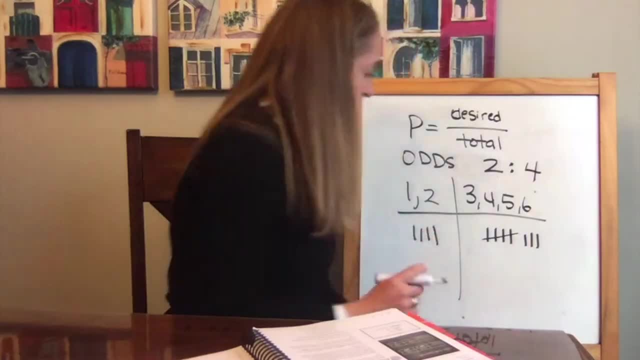 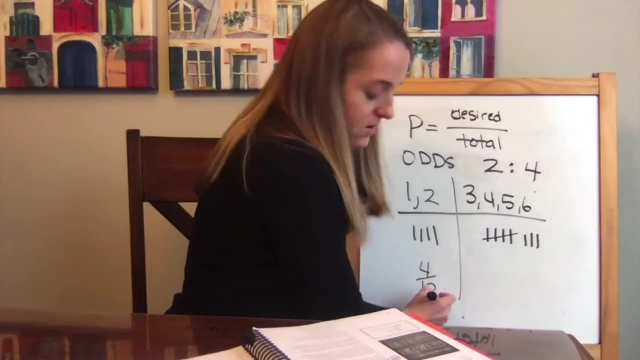 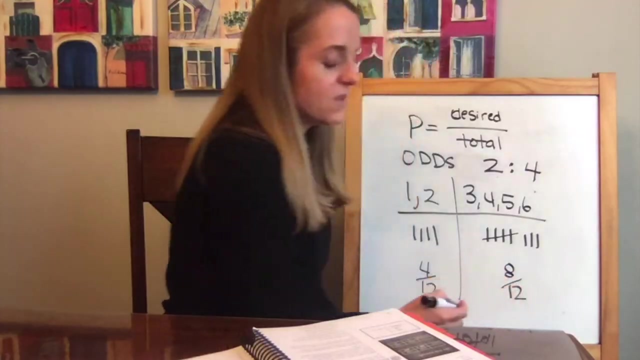 this. So this is four over 12,. 12 rolls And this is eight rolls are not yet rolls of the dice over 12.. So this reduces to one in three chances of getting a one or two, And this is two out of three chances. 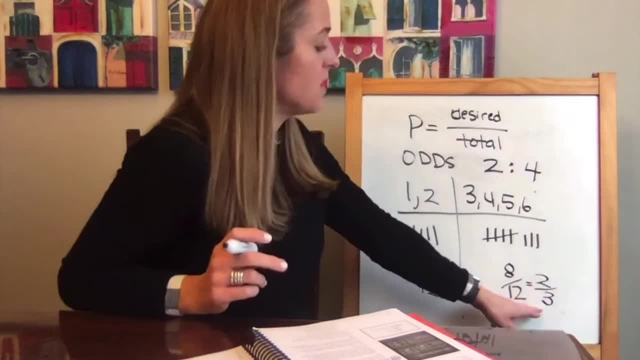 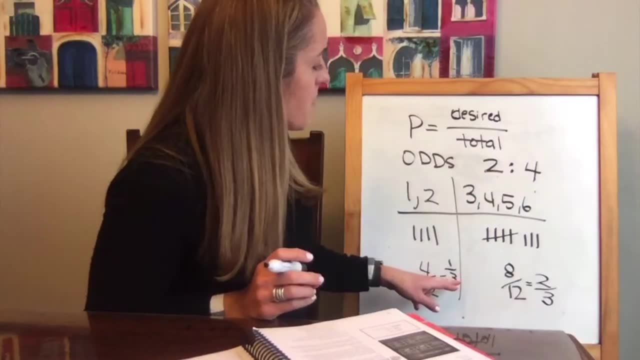 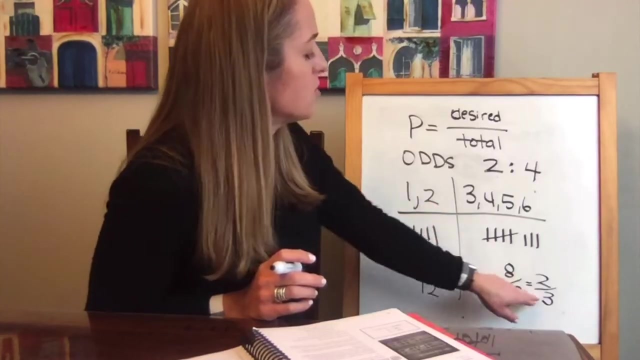 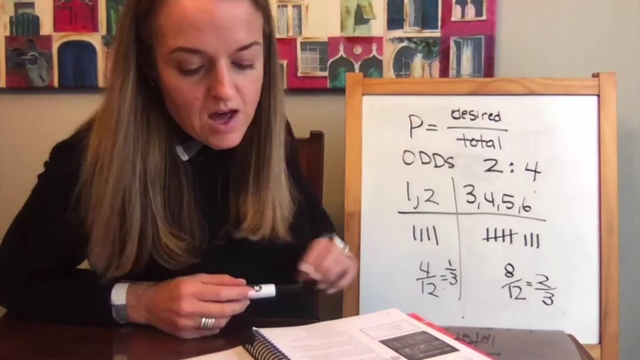 of getting one of these numbers. So the odds here are much, much better. So you see in our ratio, our odds, two to four, two numbers to four numbers, And because this is the probability, it's a one third chance of getting a one to two to two third chances of getting three, four, five or six. So both of these things can tell us a lot. Odds are usually, they're usually telling us the ratio of.